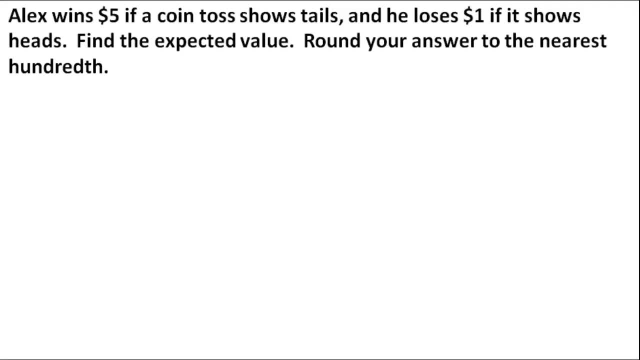 Alex is going to win $5 if he can toss a coin and it lands on tails, but he's going to lose a dollar if it doesn't. In other words, if it lands on heads, he's going to lose a dollar. We're asked to find the expected value. Okay, so the coins: we need to determine what probability there is of landing on heads or tails, and we're assuming that this one is a balanced coin, that it's not a weighted one. so it's going to land on heads. 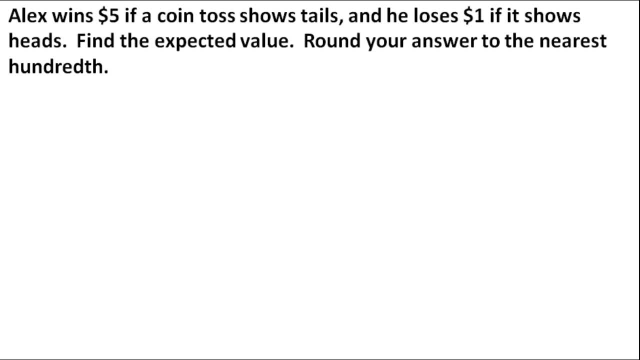 The probability is going to be the same: It's going to land on heads or tails. So when we're dealing with expected value, the way that we'll calculate this is we're going to calculate what the payout is, and the payout in this case is going to be $5. 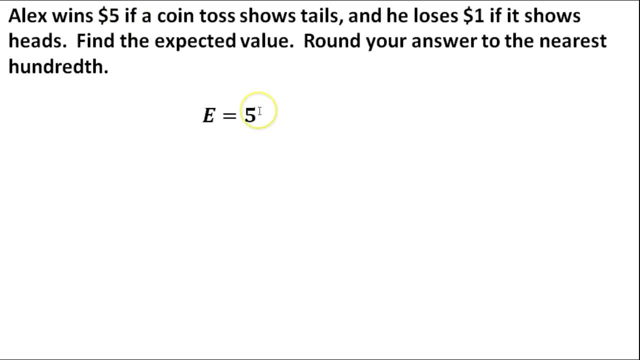 $5, so the expected value is going to be $5 times the probability that Alex is going to win that $5.. So the probability that it's going to be tails is going to be 1 half, so it's going to be 5 times 1 half. 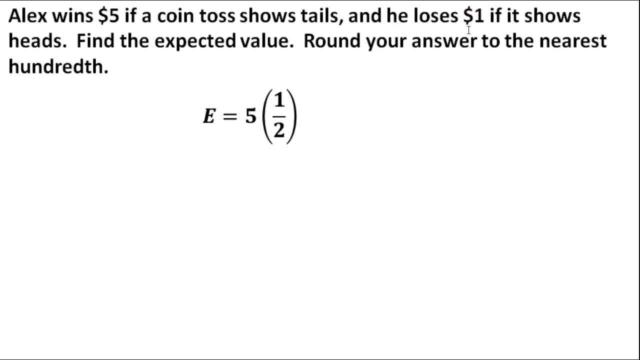 Okay, then what we're going to do is either add or subtract the other odds. Okay, and this one, he's going to lose a dollar. So because he's going to lose a dollar, we're going to subtract 1.. Okay, that's, if he was going to lose $3, he would subtract 3.. 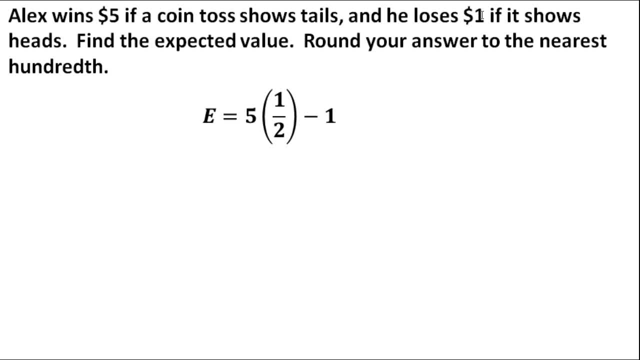 So minus 1 times the probability that this is going to occur. So he's going to lose a dollar if it shows heads. so we've got to figure out the probability of showing heads Again, that's going to be 1 half. So then we're going to multiply those two together: the 1 times the 1 half. So now what we're going to do is just simplify all of this. 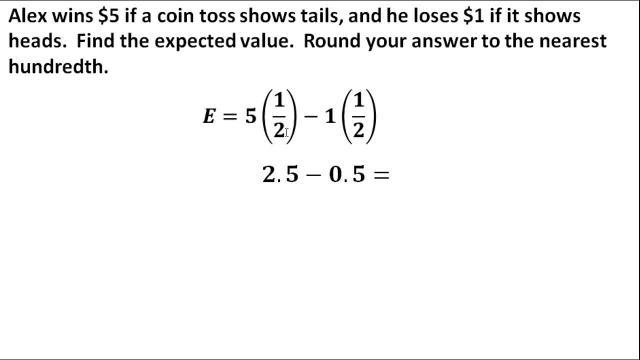 5 times 1 half is going to be 2 and a half 2.5, and then 1 times a half is just .5.. So we've got 2.5 minus .5,, which just give us plain old 2.. 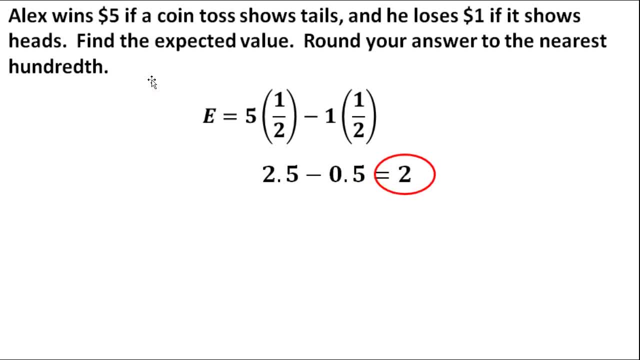 So my expected value- or Alex's expected value, I should say- is going to be 2.. Every time he flips that coin, he's expected, the more and more that he does it, that he'll end up getting 2.. 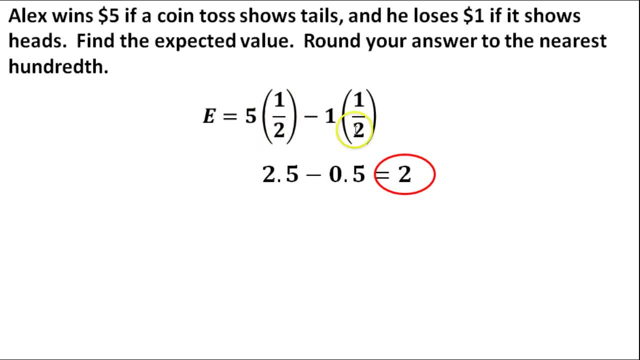 That's because he'll win $5 for every tails and he'll lose a dollar for every heads, So he's going to end up getting 2 over the long run. His expected value would be 2. So he's going to end up getting 2 over the long run.